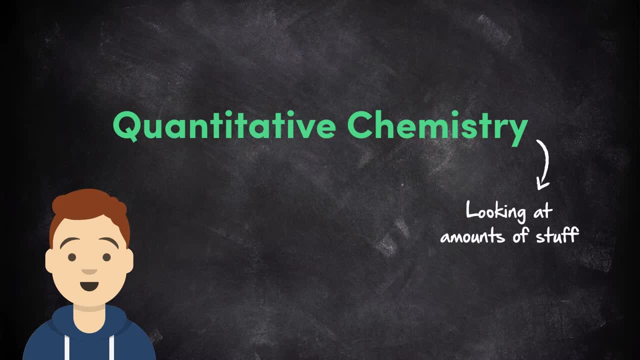 looking at and calculating amounts of stuff. Now, there's literally no way we can look at the amount of something in chemistry and not come across the infamous mole. It's actually really great that you're watching this video, because the mole is probably the most important. 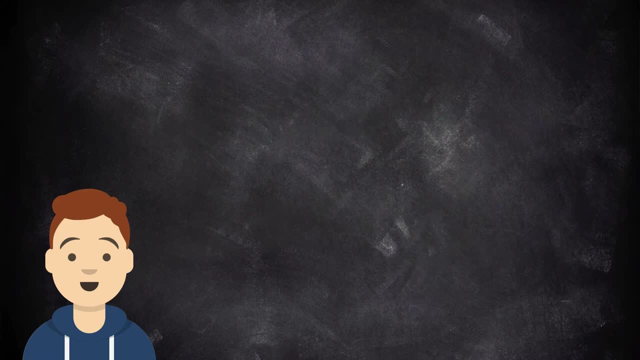 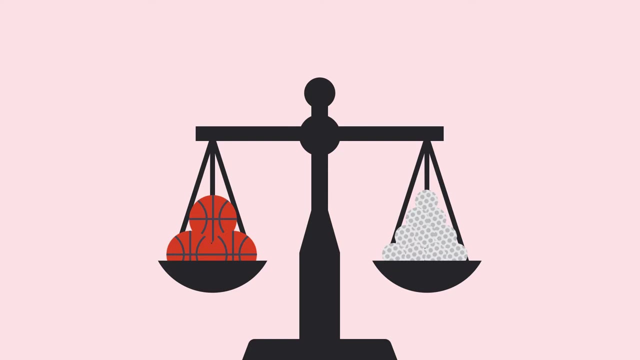 thing you'll learn for a little while. Okay, so to get in the spirit a bit, I want you to imagine having two separate collections of basketballs and golf balls weighing 10 kilos each. Now think about the difference in the amount of balls between the two You. 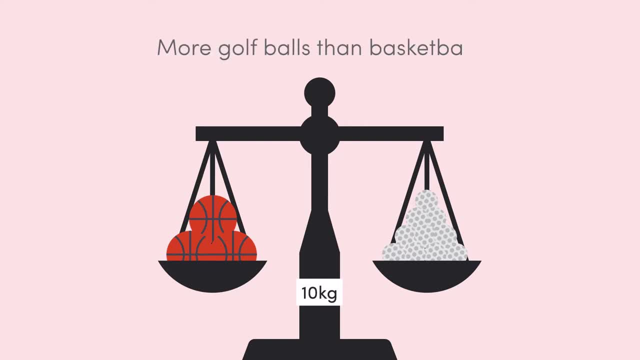 don't need to be a genius to know that there'll definitely be more golf balls than basketballs- 218 compared to 16, in fact- And this is the case Even though the total masses are equal to each other. you can play a lot more games. 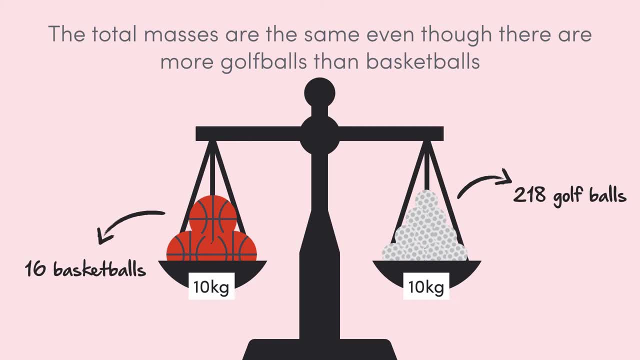 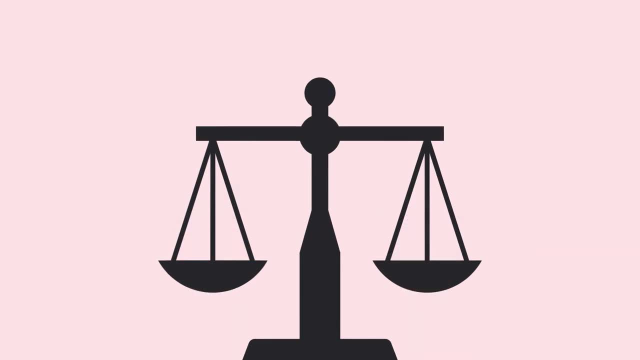 of golf than you can basketball, assuming you don't lose heaps of balls in the water, like I did when I tried. So why did I bring up this example? Well, because this exact same idea exists in chemistry. when we deal with particles of different sizes, We're easily 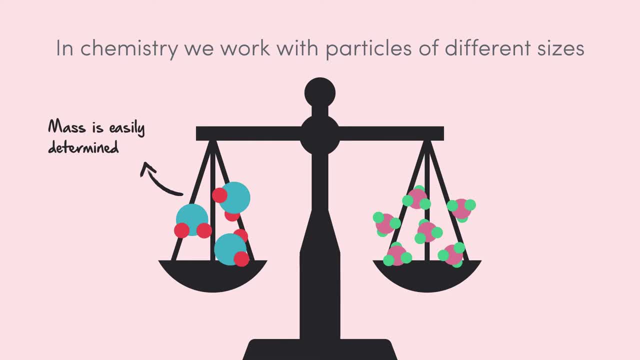 able to determine mass by weighing something. but measuring an amount of substance by mass doesn't directly give us the amount of particles in that substance. 218.. So we're able to determine mass by measuring the number of particles in a substance. So we'll start by looking at the number of particles in a substance. 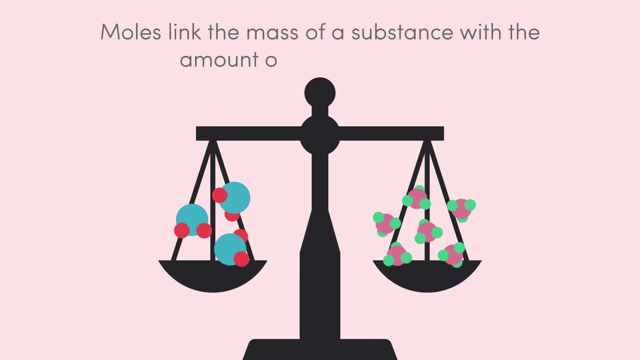 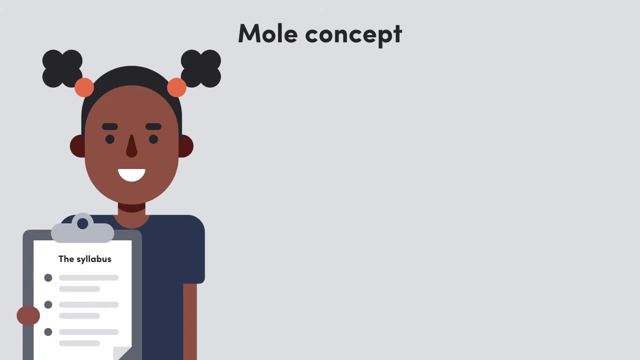 And this is where moles come in, to link the mass of a substance with the number of particles in it. You can check out the attached syllabus- dot points on the video page to see where all of this content comes from. So we'll firstly look at what moles actually are and from this we'll do a couple of conversions. 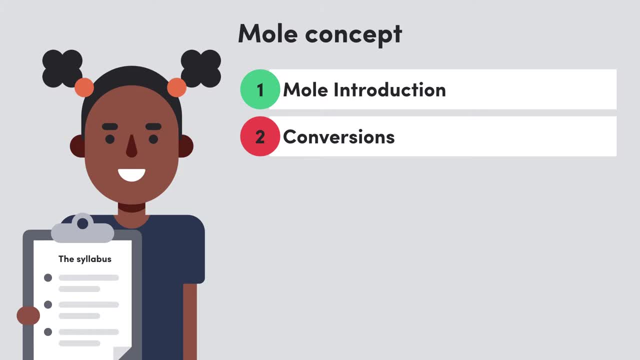 between an actual number of particles and number of moles of that particle we have. We'll then put on our thinking caps and actually try to make sense of the theory surrounding the mole concept and how this ties into the molar masses of different substances. 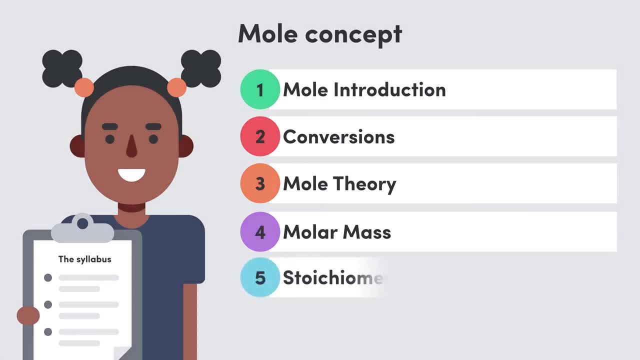 And finally, we'll link this all, really briefly, into the idea of stoichiometry, Which sounds really complex, but trust me, it isn't. So with all that to do, let's get cracking with an introduction to the concept of moles. 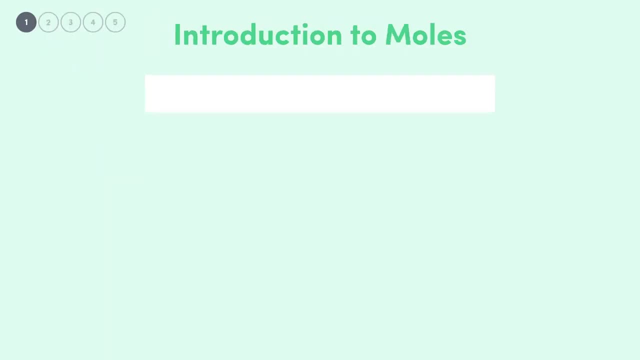 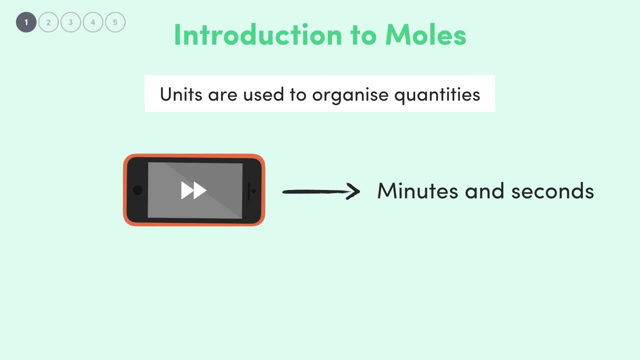 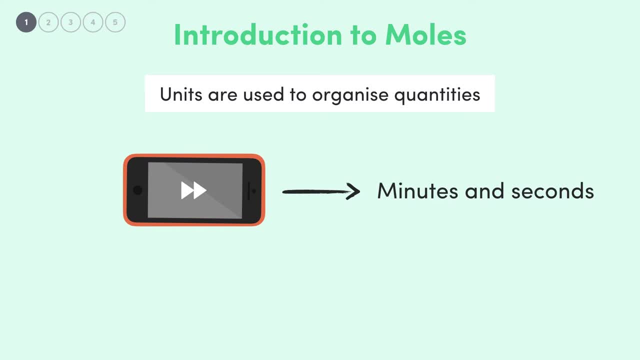 But if I were to tell you that at the time of recording this video I was born 11,987,640 minutes ago, you'd think I was a right weirdo. And that's because when you're asking the age of somebody, you'd typically expect the answer to be in years. 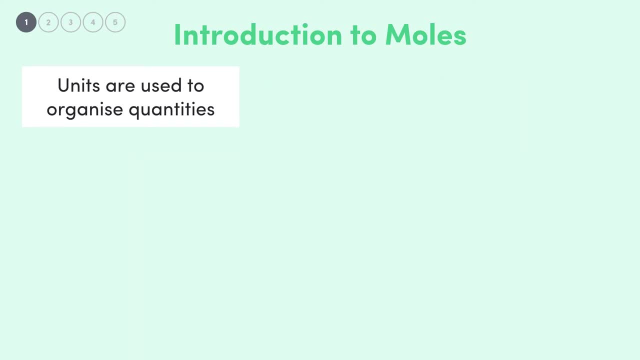 Now I'll leave it to you to figure out how old I am in years, but chemists are always dealing in numbers of atoms and molecules and, if you think about it, this could get pretty tricky aswell. these are so tiny and there are so many substances we want to measure Even a small amount of. 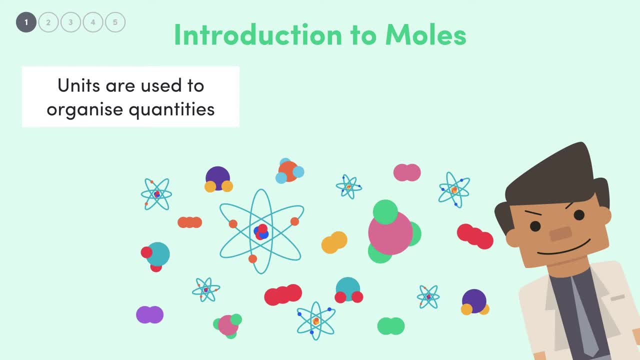 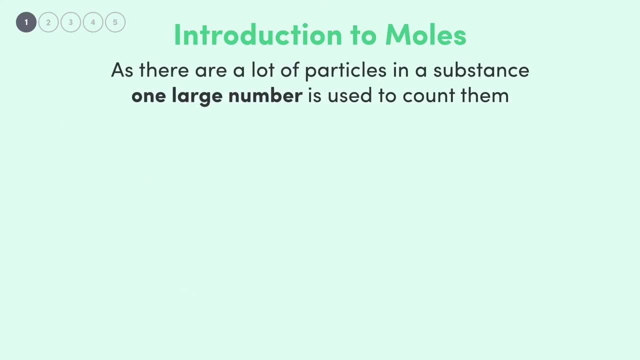 matter contains trillions of atoms, So it makes sense that we would use a large number to help us count the number of atoms or molecules in a substance. That specific number, 6.022 times 10 to the power of 23,, is known as Avogadro's constant. It gives us the number of particles. 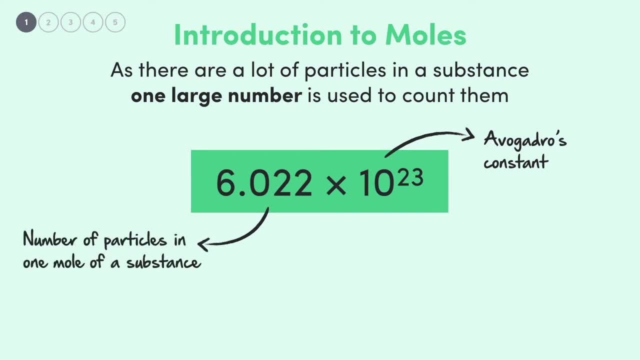 in a mole. Don't worry about needing to remember this, it's going to be given to you on your formula sheet. So, in other words, no matter what substance you're talking about, we say a mole of it is 6.022 times 10 to the 23 particles of it. So now that we know what, 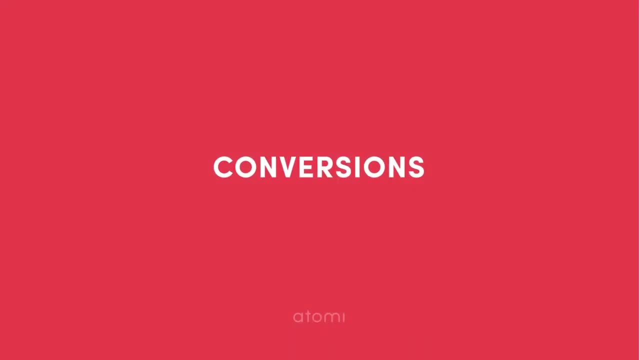 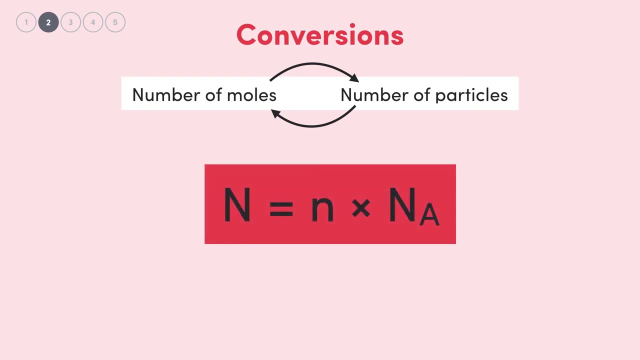 a mole is, it makes sense that we should be able to convert between an actual number of particles and number of moles. We know that there is Avogadro's number of particles in one mole. so converting from number of moles, which is written as a lowercase n, to particle. 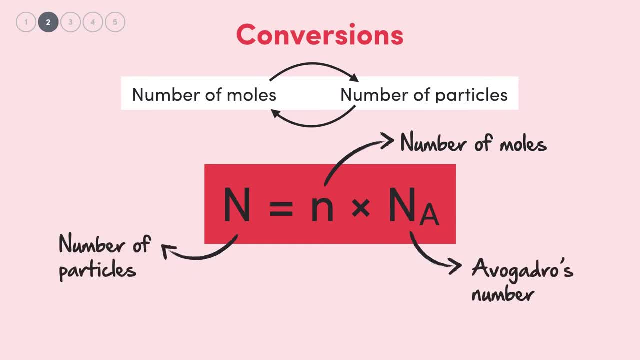 number. we simply multiply. So we have 6.022 multiplied by Avogadro's number, which is given by this symbol, And it's made pretty obvious by this little a here, Of course, the opposite direction applies too. Converting from number of particles to number of moles requires division by Avogadro's. 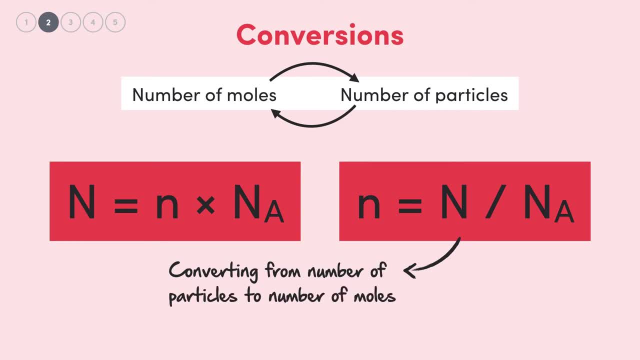 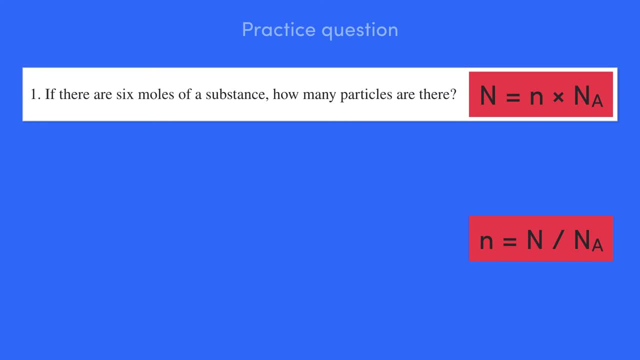 constant. OK, great. So let's do a couple of examples. There's 6 moles of a substance. How many particles is this? Well, 6 multiplied by Avogadro's constant gives us 3.613 times 10 to the power. 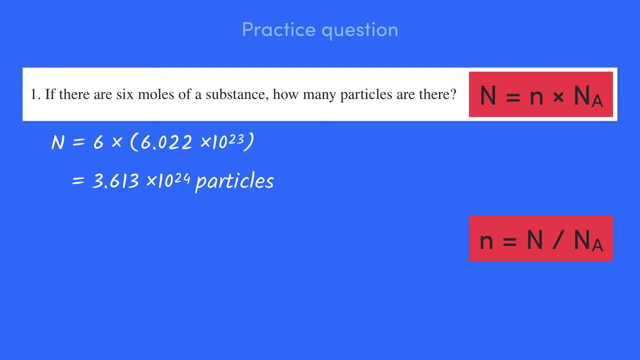 of 23.. So we have 6.022 multiplied by Avogadro's constant, which is written as a lowercase n to particle, minus 10 to the power of 24.. Alright, if I have 11 times 10 to the power of 23 atoms, how many moles do I have? 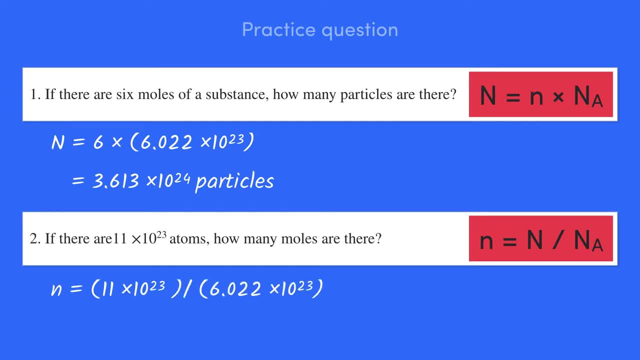 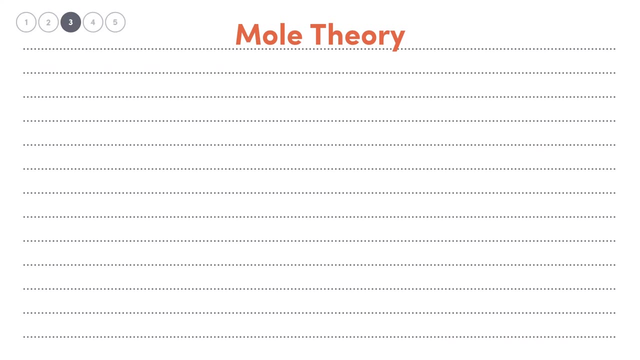 Well, 11 multiplied by Avogadro's constant becomes 1.83 moles- Easy peasy. So I can almost hear you guys say: yeah, it makes sense that we use a really big number to count molecules and atoms. but 6.022 multiplied by 10 to the power of 23 seems a bit random. 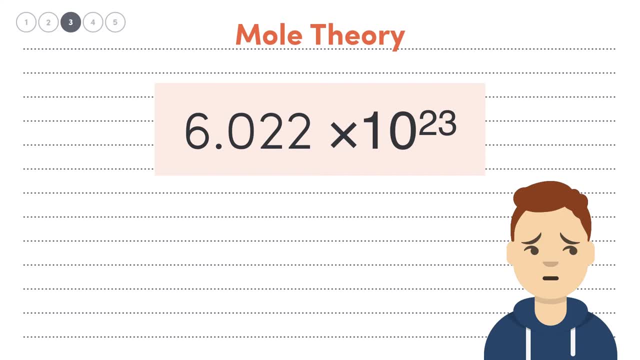 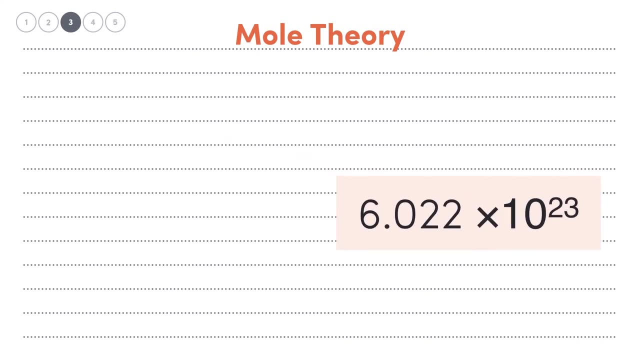 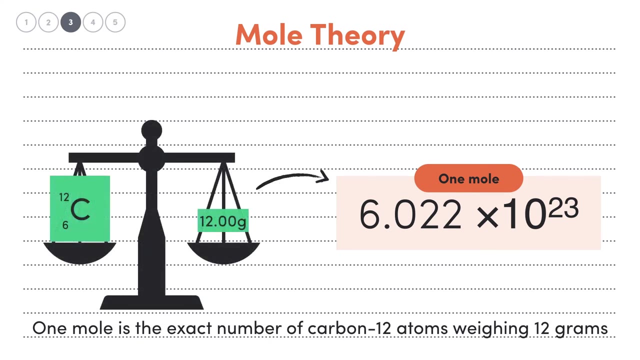 doesn't it? Well, you're right, It is a pretty weird number, but it's like that because it's been specifically designed by chemists to be the most useful number possible. One mole is defined as the exact number of carbon-12 atoms weighing 12 grams. Carbon-12 is chosen as the reference point for most things. 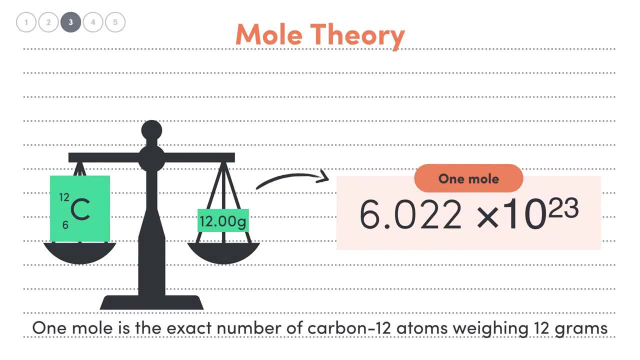 to do with comparing elements, and so this is no different. This is so useful, since we can use this to relate the mass of a substance to the amount of moles. The atomic weight or relative atomic mass on the periodic table is an atomic mass unit, AMU- and tells us the mass of one mole. 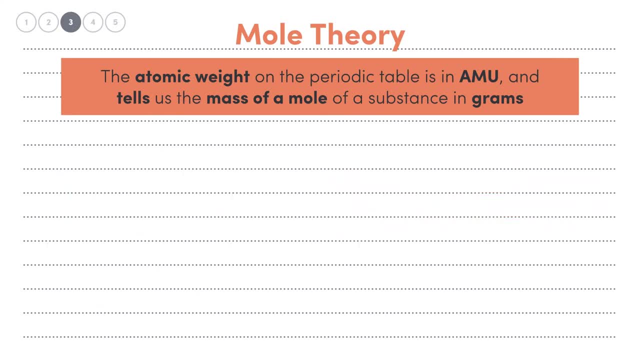 of a substance. So, looking at our atomic weight, we know that hydrogen has an atomic weight of 1.01 atomic mass units, meaning that one mole of hydrogen atoms will weigh 1.01 grams, In other words, 1.01 grams of hydrogen. 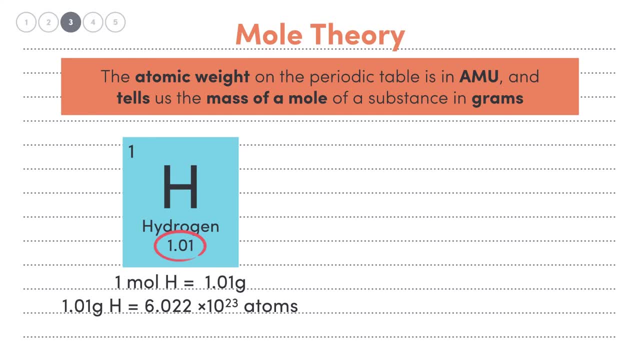 is the atomic weight of a substance. Hydrogen has 6.022 times 10 to the power of 23 particles in it. Furthermore, oxygen has a relative atomic weight of 16.00 atomic mass units, meaning one mole of oxygen atoms will weigh 16.00 grams, and so on. 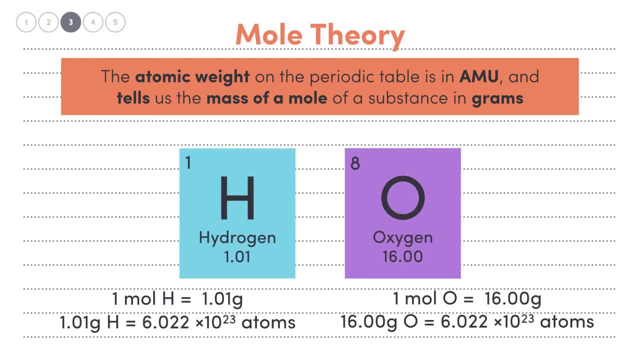 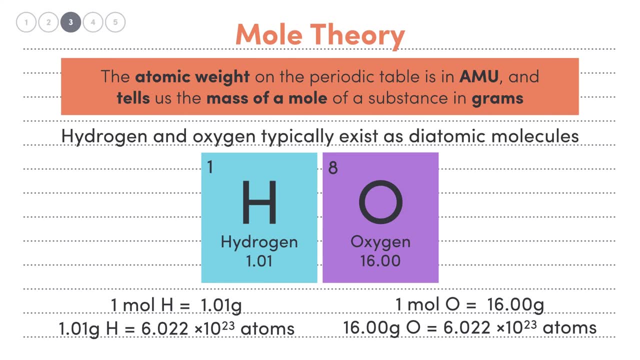 Just a little point to notice here. Hydrogen and oxygen typically exist as diatomic molecules, which is just a molecule made of two atoms of the same element. So if we were asked to find the molar masses of hydrogen or oxygen gas, we'd need to multiply these values by two. 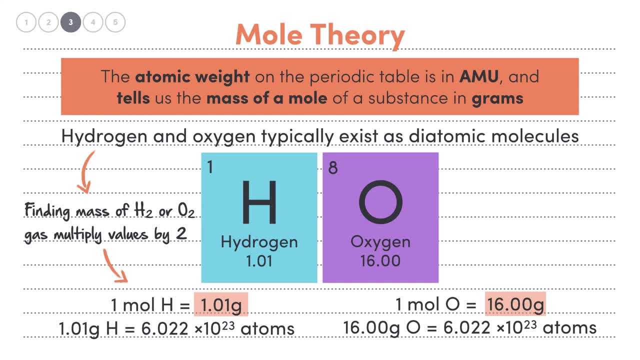 If you guys are at all unsure about how we get these numbers for our relative atomic weights, that's all good. Just go back and check out the past videos on relative mass. So to tell the mass of one mole of an atom, which is called the molar mass, 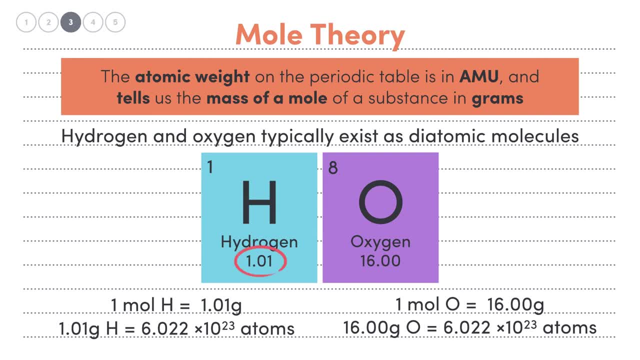 it's literally as easy as reading the atomic weight of the corresponding atom off the periodic table and writing this in terms of grams. Again, if this is seeming totally new to you and you want to check it out in more detail, head back to the video called Relative Mass, Part 2.. 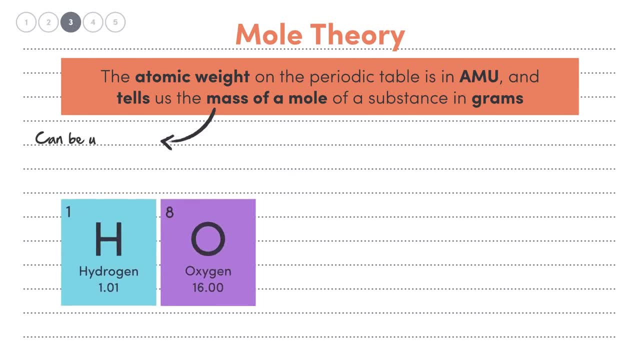 We are then able to use this same idea when talking about molecules, as these are just combinations of atoms. For example, one molecule of water is made up of two hydrogens and one oxygen, meaning its molecular weight is equal to two times the atomic weight of hydrogen. 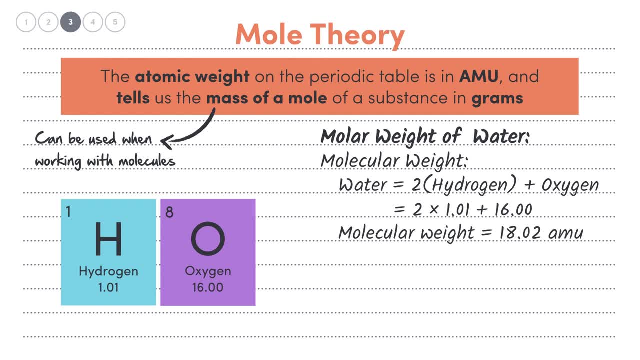 plus the atomic weight of oxygen, which equals 18.02.. That means that one mole of water molecules will weigh 18.00 grams. Okay, I think it's important here to clear up a little bit of terminology that can be a bit confusing. 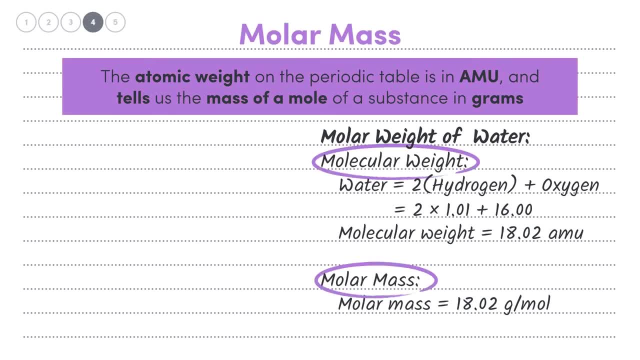 The difference between molecular weight and molar mass. Molecular weight is simply the combined atomic masses of all the atoms in a molecule. written as a number, This is obviously going to be a tiny mass, and so it's in atomic mass units. But the key thing is that the molecular weight is equal to the mass in grams of a mole of that molecule. 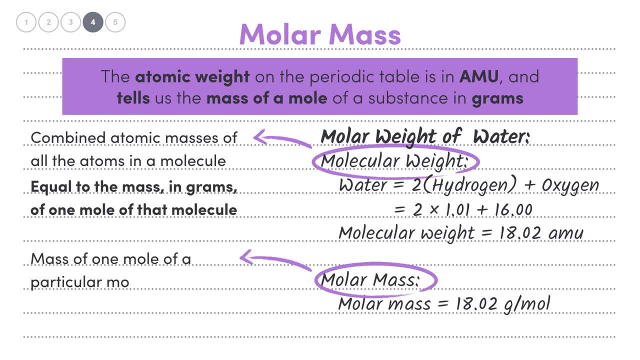 So to convert this into a molar mass, MR, which is the mass of one mole, of a particular molecule, we simply write in the units grams per mole. after It's really that simple, Using our molar mass will become really useful in our mass-to-mole calculations, which we'll dive into in another video. 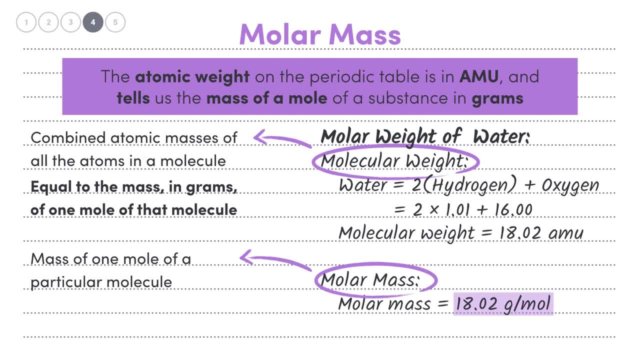 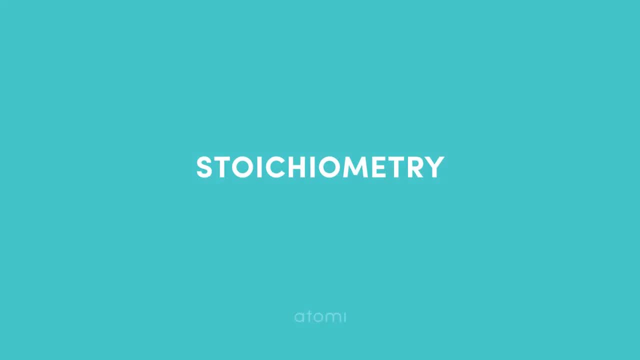 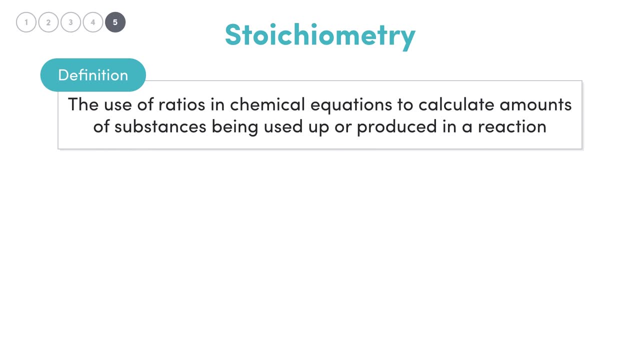 So definitely tune in for that. So what on earth do moles have to do with our chemical reactions? Well, this is where we introduce the term stoichiometry. Simply put, stoichiometry is the idea of using ratios in chemical equations to calculate amounts of substances being used up. 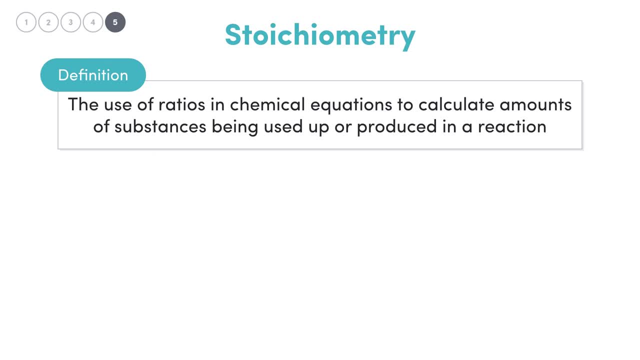 or produced in a reaction. So just looking at our reaction to produce water before we thought of the numbers. here is referring to the number of atoms involved in the reaction, But of course, since moles are just a way of counting atoms, the same ratio will apply to moles as the amount of atoms. 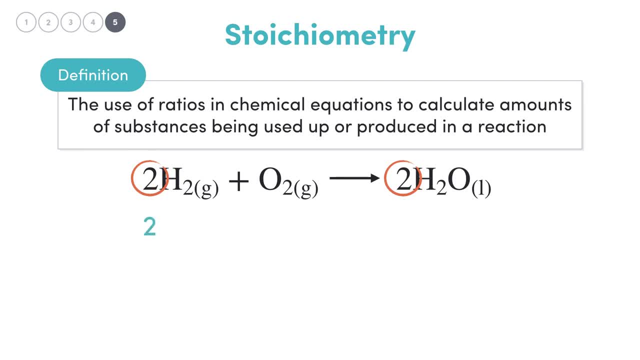 So we can now read into this equation. So we can now read into this equation. read into this is telling us that for every two moles of hydrogen gas and one mole of oxygen that react, two moles of water molecules are formed. these are known as the molar ratios of this equation. we can then use the same ratio.